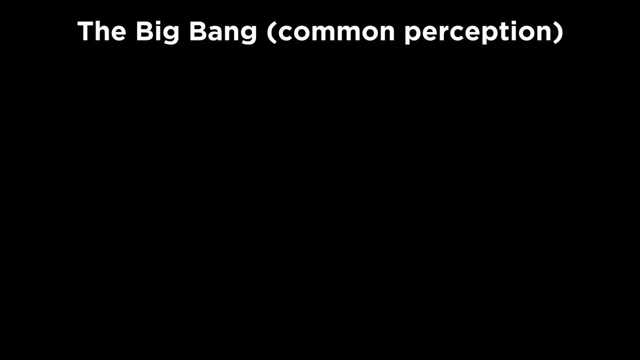 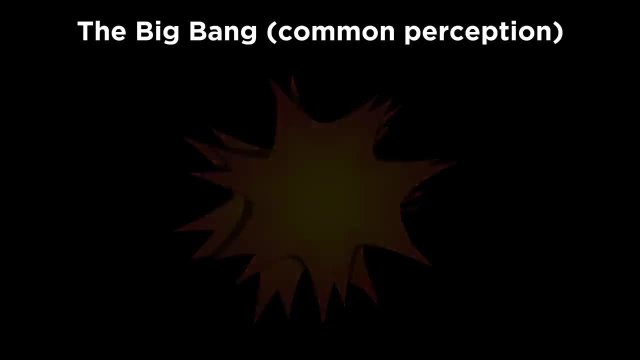 principles in physics and astronomy. When most people imagine the Big Bang, they think of a loud kaboom, a cartoon explosion graphic and the present-day fully formed universe spilling out of it, with a comet and the planet Saturn and other complex objects. 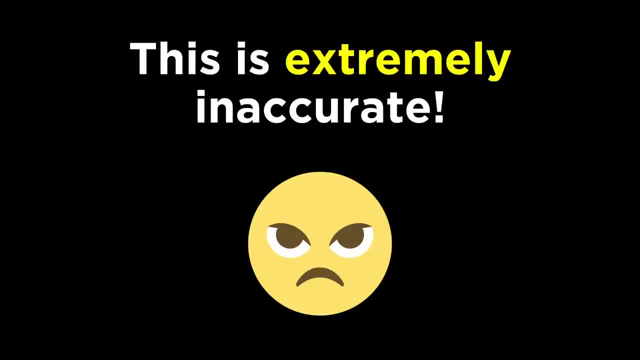 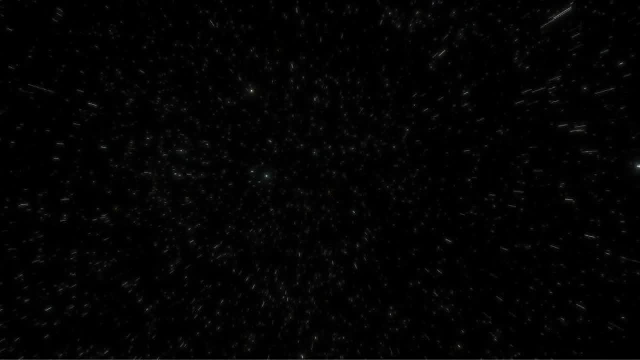 This would indeed be impossible to believe and in fact it could not be further from the truth. In this tutorial, we will describe in a basic way our current model for the birth and early development of the universe, as understood by modern science. 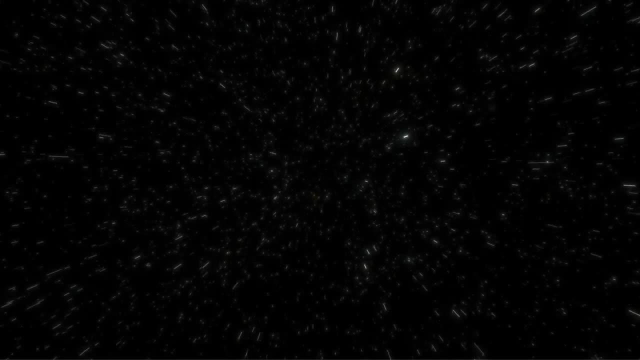 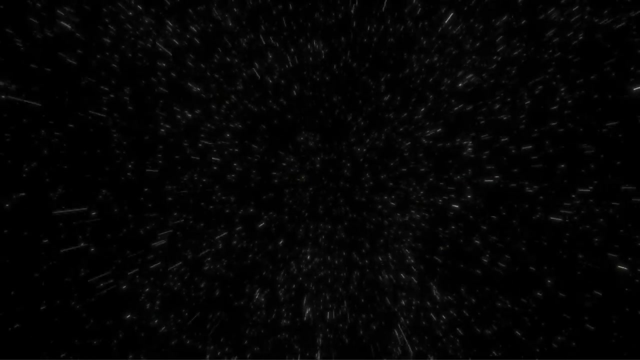 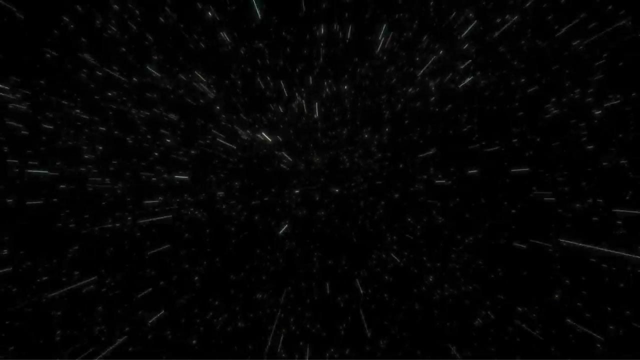 So let's get started. Unfortunately, we will not yet be ready to discuss the evidence that supports this model, because understanding that evidence will require a discussion of galaxies and many other objects that we will get to later in the series. So for now, try to simply take this model at face value, and I promise that later on. 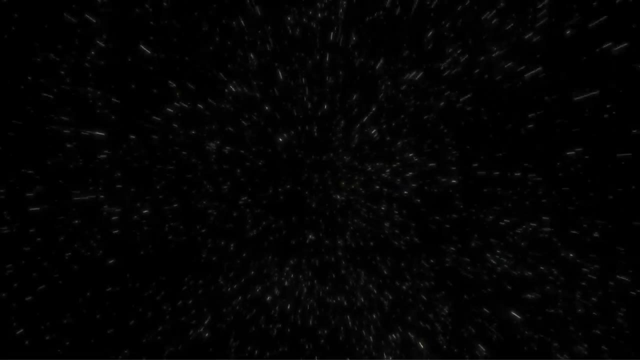 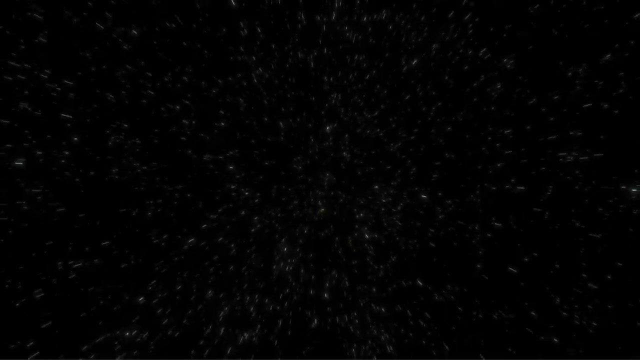 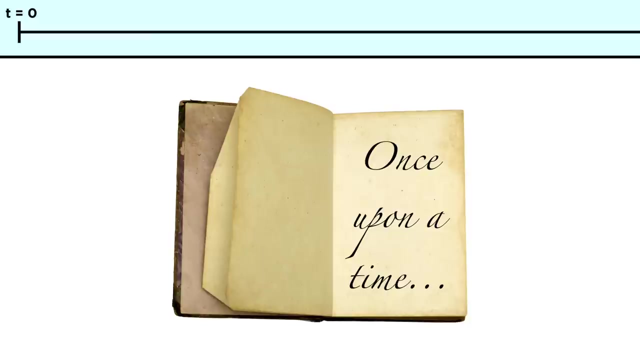 we will examine several independent threads of evidence that all corroborate this model of the universe to great precision. So now let's start at the beginning. To be fair, at present we don't know what happened at the beginning. By the beginning we mean: t equals zero, the first instant. 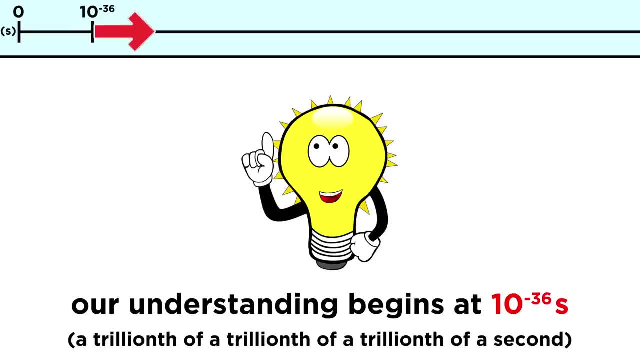 Our understanding begins to take shape at around ten to the negative. thirty-six seconds after the Big Bang. That's a trillionth of a trillionth of a trillionth of a second. From that moment forward, we start to have an increasingly solid grasp of how things. 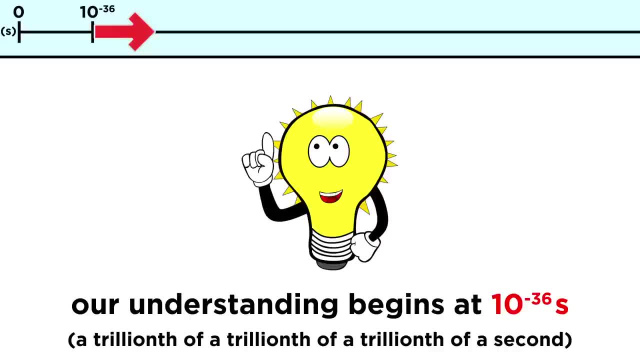 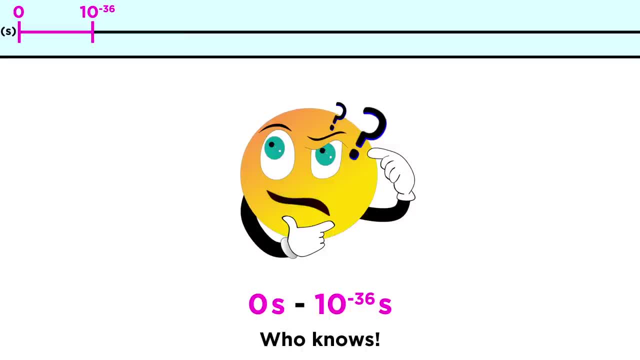 must have gone, Which is pretty darn impressive when you think about it. As for the imperceivably small increment of time before that, we must admit that our current models just don't work. We will still talk about this earliest period here, but, to be clear, it will be largely 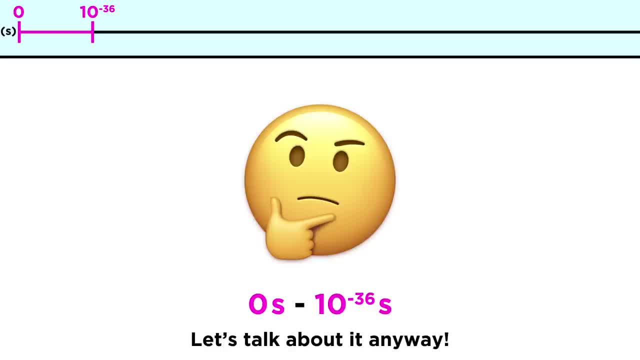 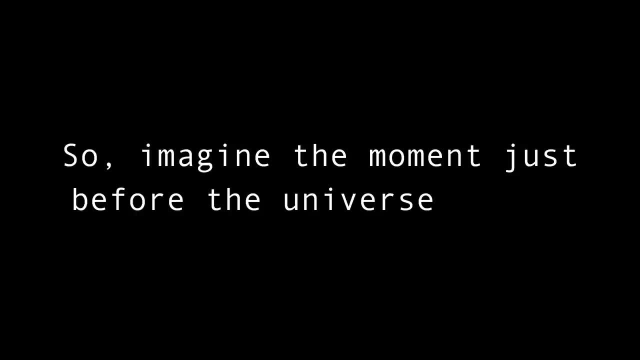 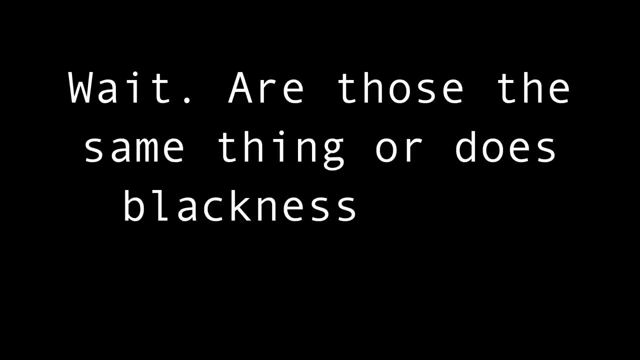 speculative, including some of my own personal conjecture, But don't worry, we will quickly get back to the real science. So imagine the moment just before the universe began: Nothingness, Complete blackness. Wait, are those the same thing, or does blackness count as something? 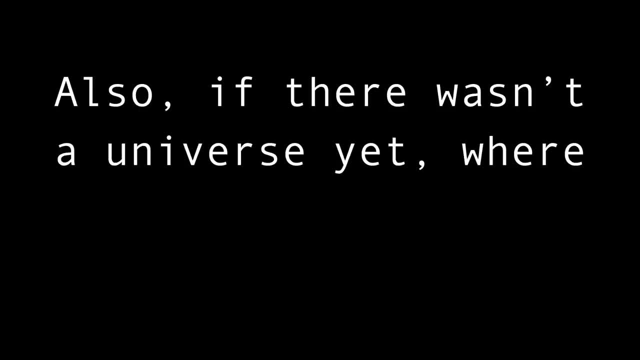 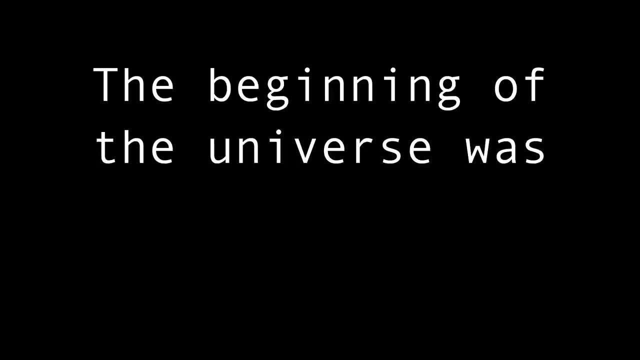 How do we show nothingness? Also, if there wasn't a universe yet, where are we sitting right now to watch this? Hmm, well, what was there before the universe? The beginning of the universe was the beginning of time, so does a question that includes 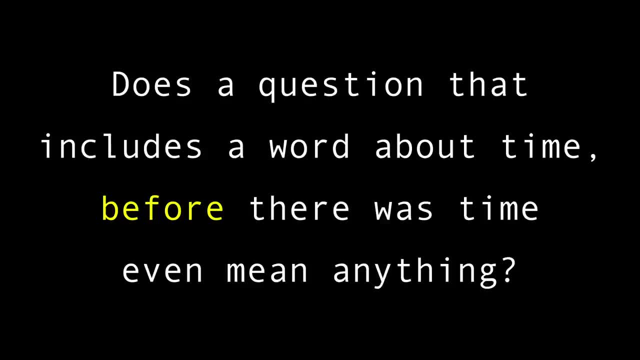 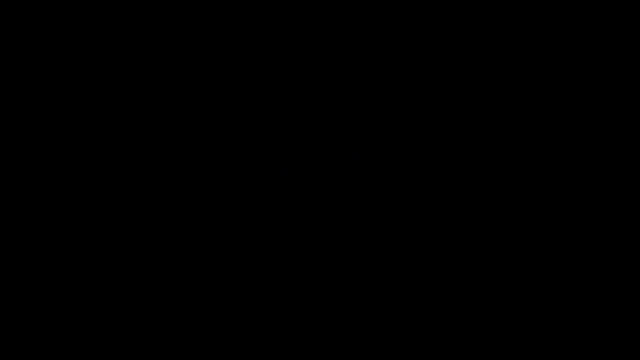 a word about time before there was time even mean anything? Wait before there was time? oh man, I did it again. I'm already exhausted. Let's just start at the first moment. I'm already exhausted. Let's start at the first moment and picture blackness, since that's kind of the best. 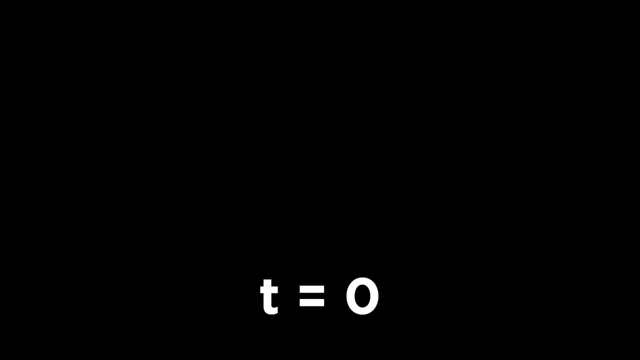 we can do Now? the first thing: time zero, Freeze the clock. A single point: the uncaused cause. How could this have happened? Let's first recall some things about the Heisenberg uncertainty principle. This tells us that when looking at complementary variables like energy and time, the more 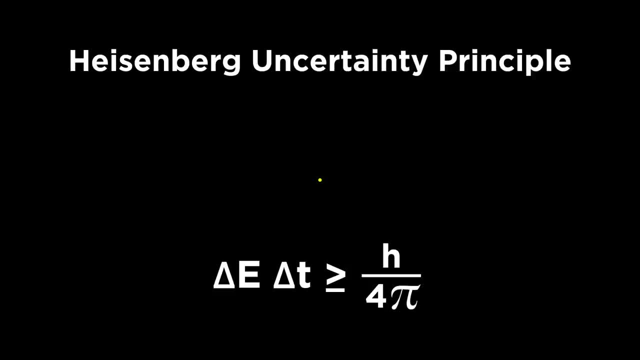 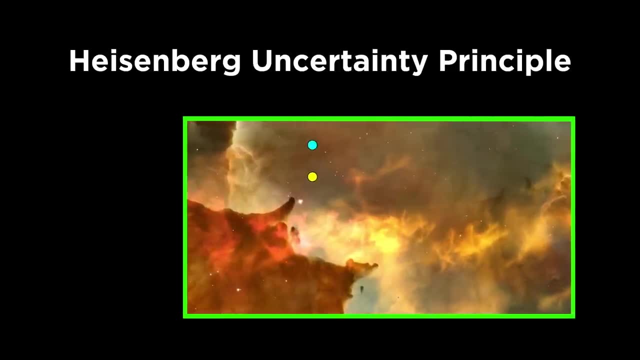 certainty associated with one, the less certainty that can be associated with the other. This is what allows for quantum fluctuation, The very real and very measurable phenomenon by which particles pop into and out of existence, all over the universe and at all times. 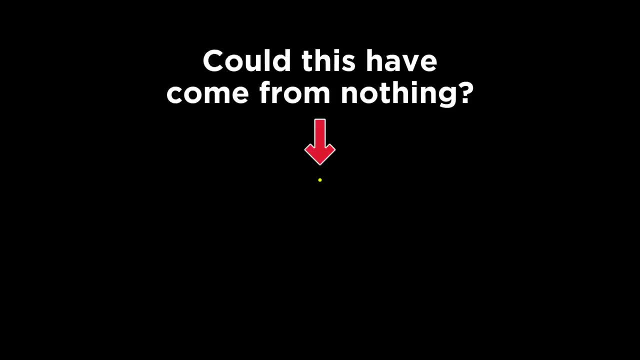 This means that the idea that something could simply appear is actually not without precedent. Of course, to go from virtual particles to the entire universe is quite a leap for a number of reasons, but if you really think about it, with nothing else in existence yet, 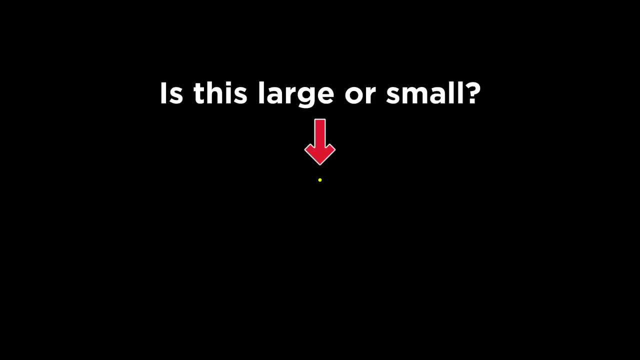 to be compared to. would this fluctuation have been large or small? Is it a lot of energy or a little? In comparison to what? precisely What if, taking into account both positive and negative energy, the net energy is very close to zero? 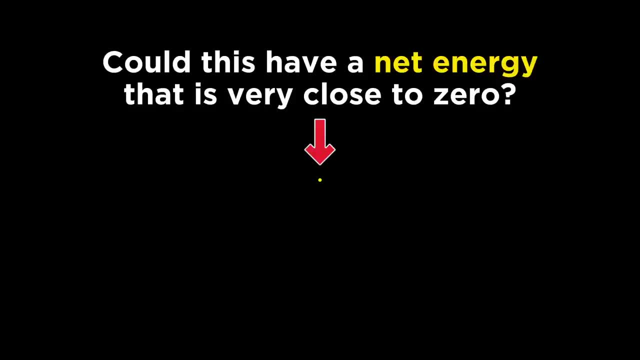 Then the entire universe could be regarded as a quantum fluctuation borrowing energy. it will pay back later. If we take for granted that, without any other frame of reference, a quantitative amount of energy appearing from nothing can be of any arbitrary amount, then we are acknowledging 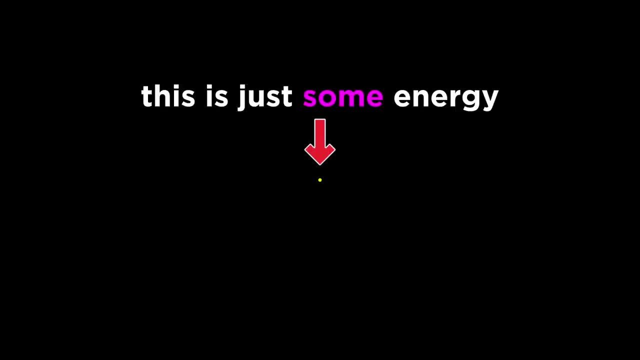 that the appearance of some energy is not Energy from no energy is the only thing we must explain. It is the emergence of an initial duality: plus and minus, yes and no. Whatever you want to call it, It is not planets and stars tumbling out of a kablooey graphic. 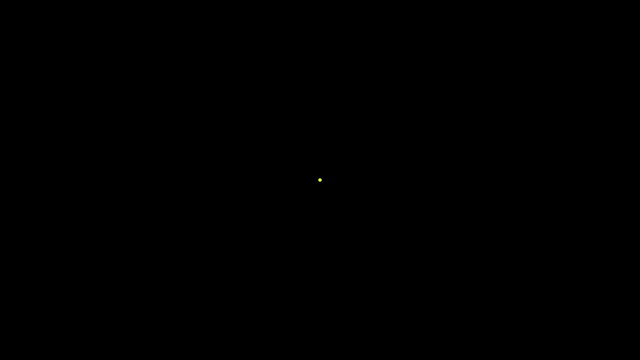 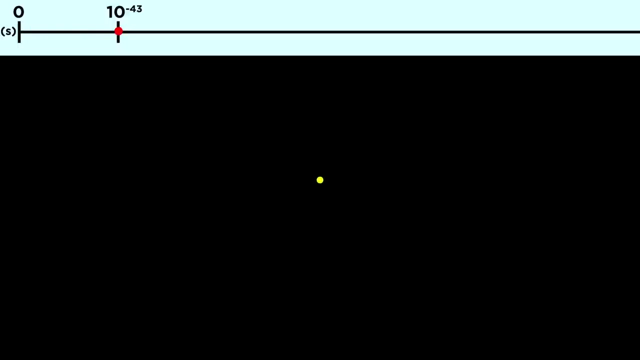 It is the emergence of the simplest possible thing, that is, a thing rather than no thing. Everything else follows from there. Now we get to ten, to the negative forty-three seconds after the big bang. What do we know This time? Still not much. 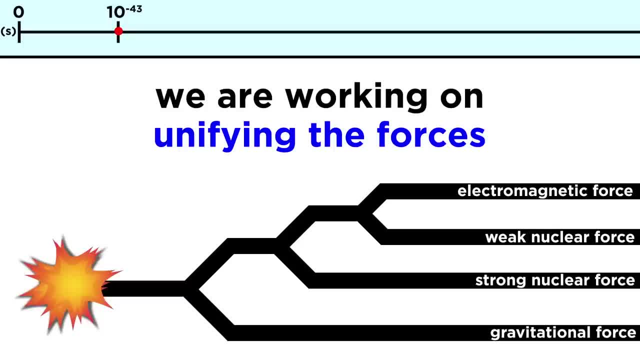 But if we recall some things about the standard model of particle physics, experiments in particle accelerators have allowed us to begin the incredible task of unifying the four fundamental forces. These are the electromagnetic force, the weak nuclear force, the strong nuclear force and 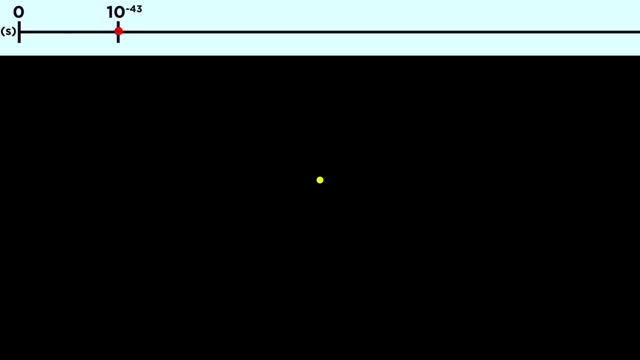 gravity. In that earliest period that we know almost nothing about, also called the Planck epoch, the temperature of the universe must have been over ten to the thirty-two kelvin, which is nearly a billion trillion trillion degrees- far too hot for familiar particles to exist. 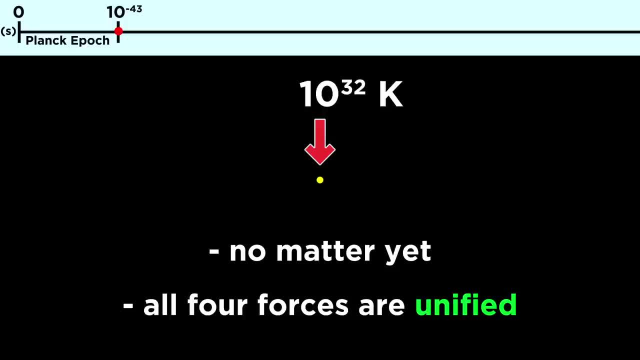 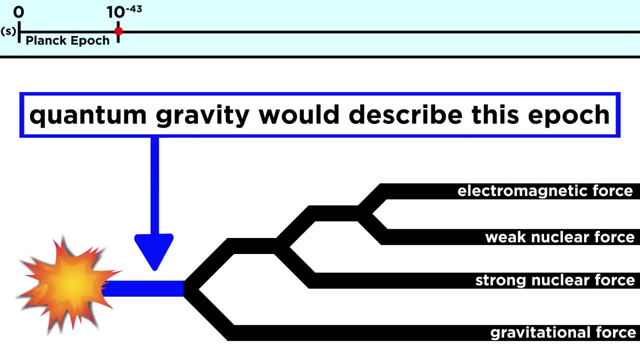 and all four forces must have been unified into one single force. The search for quantum gravity is the search for the quantum particle that would mediate this singular force. thus it is sometimes called the search for the theory of everything. Particle accelerators can't yet achieve this incredible energy. 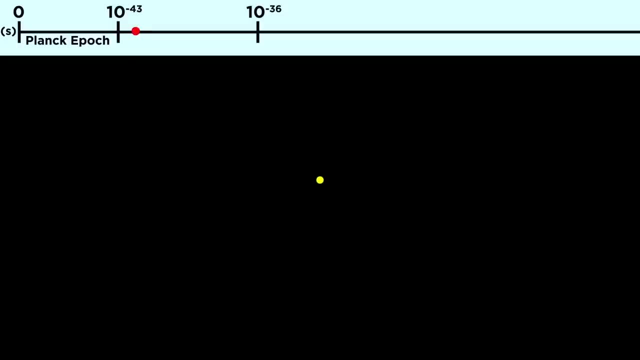 So we must hope for bigger and better technology, But in the next epoch, from ten to the negative forty-three seconds until ten to the negative thirty-six seconds, also called the grand unification epoch, temperatures cooled down to ten to the twenty-nine kelvin. 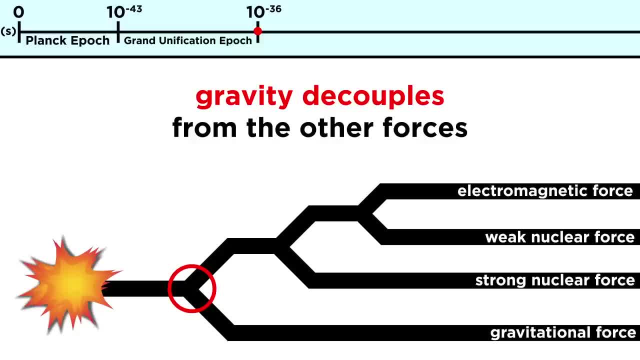 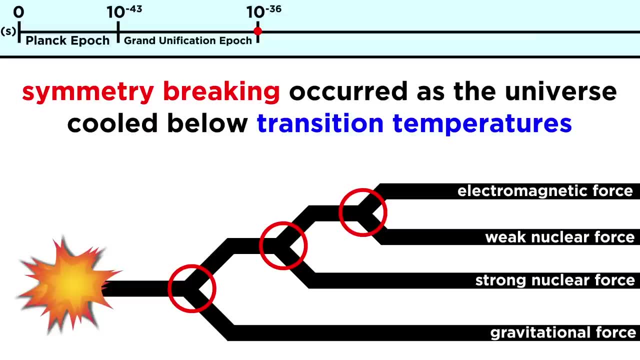 This allowed for gravity to decouple from the other three forces, which can be collectively referred to as the electrostrong force and which we believe could potentially be described by a grand unified theory. This act of forces breaking off from other forces is the result of symmetry breaking. 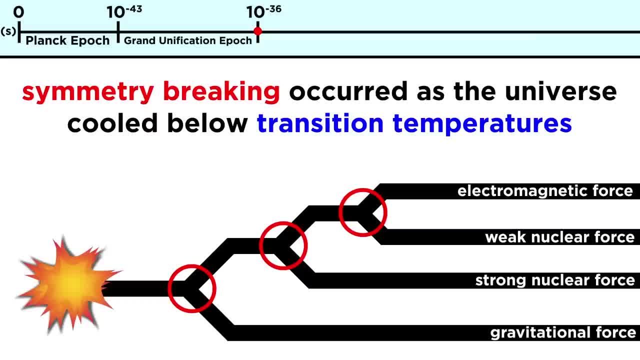 a phenomenon that can occur when extreme temperatures cool below certain transition temperatures. In this way, we can understand that all the disparate fundamental particles in the universe were once part of the same thing that only manifested as different objects as a result of a series of successive symmetry breakings while the universe was changing. 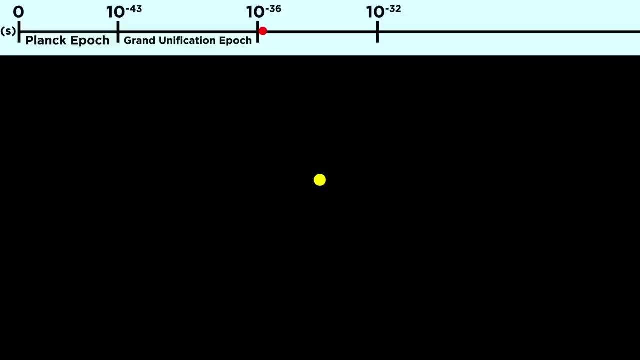 The universe cooled. Next we enter the earliest era for which theoretical physics has some reasonable basis, taking place from ten to the negative thirty-six seconds until ten to the negative thirty-two seconds after the Big Bang. This is called the electroweak epoch. 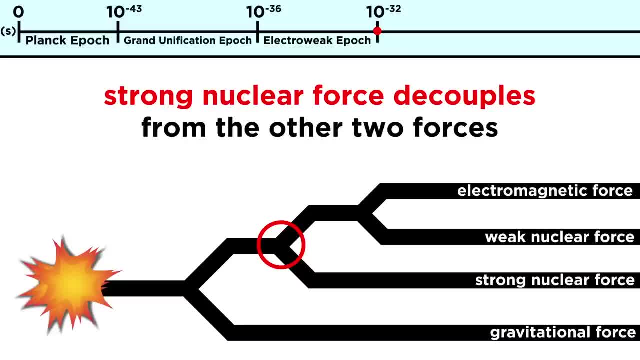 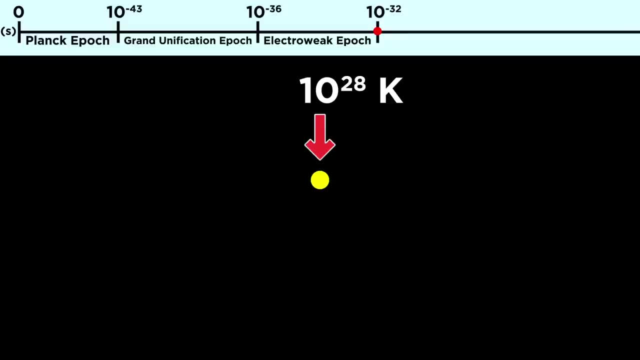 It is marked by the decoupling of the strong nuclear force from the electrostrong force, leaving only the electromagnetic and weak nuclear forces together, Which we call the electroweak force. This is possible now with the universe having cooled to a frosty ten to the twenty-eight. 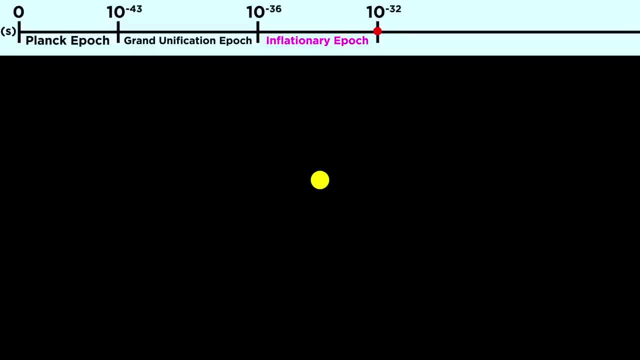 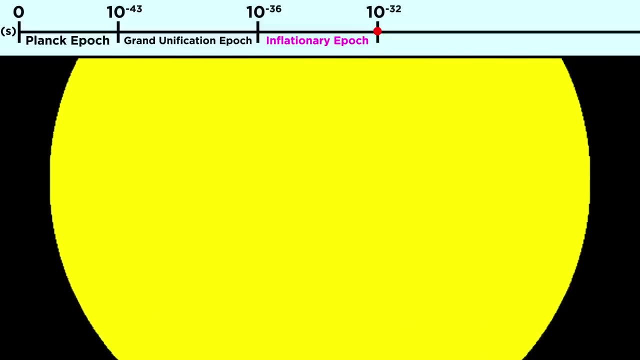 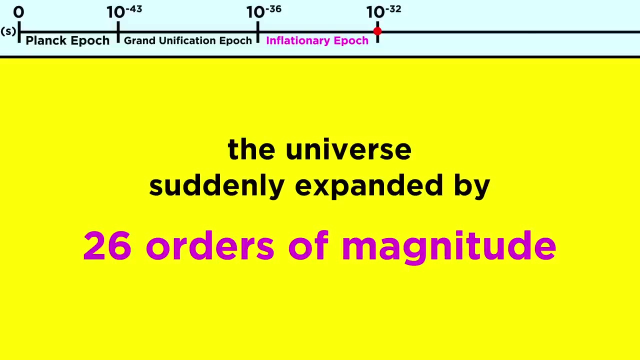 kelvin. Roughly concurrent with the electroweak epoch is what we call the inflationary epoch. This was a brief period in which the universe expanded by an incredible factor around twenty-six orders of magnitude, triggered by the separation of the electrostrong force into the strong. 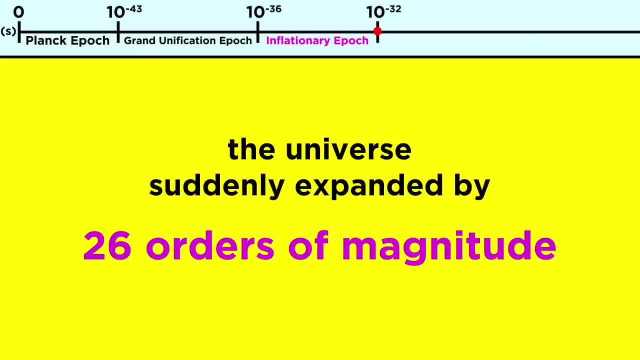 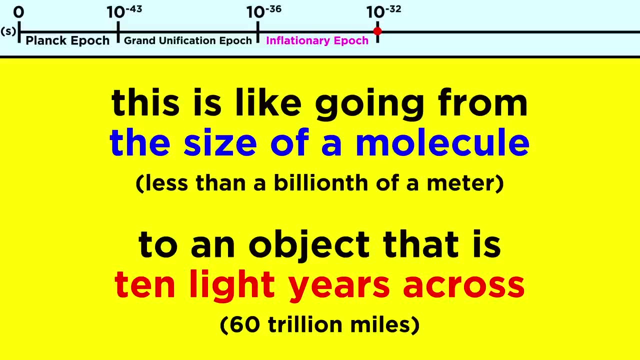 nuclear force in the universe. We don't know the precise size of the universe before and after this phase, but the magnitude of the expansion would be like inflating something the size of a small molecule up to something ten light years across or about sixty trillion miles. 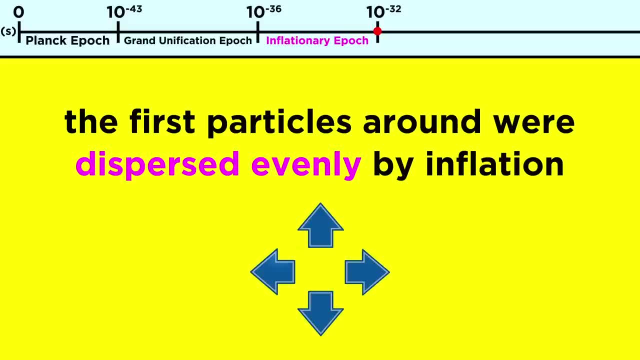 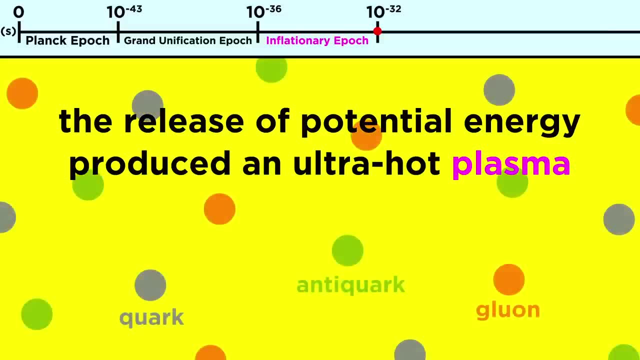 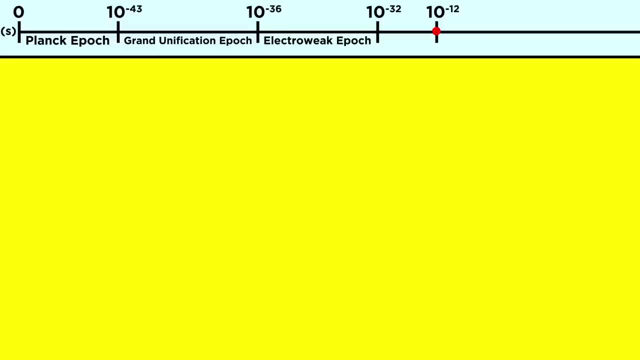 This nearly instantaneous expansion dispersed the earliest fundamental particles around this much larger volume quite evenly, after which the immense potential of the future, immense potential energy from the inflation was released, producing a hot plasma of quarks, anti-quarks and gluons Plotting along to around ten, to the negative twelve seconds, or one trillionth of a second. 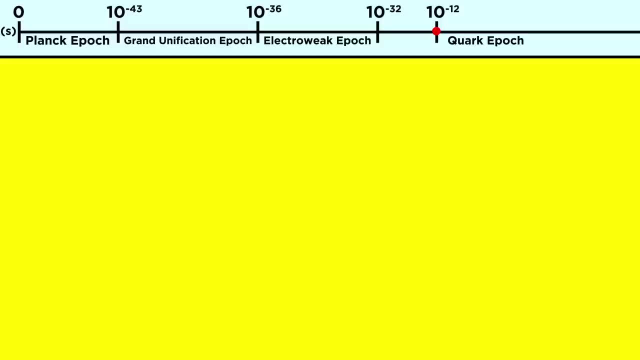 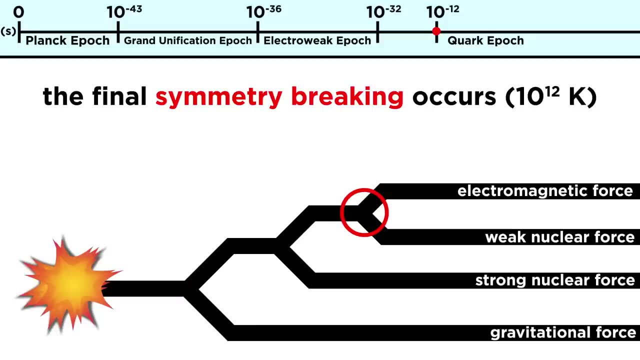 after the big bang we enter a period called the quark epoch. Here things have cooled enough for the third and final symmetry to break, decoupling the electromagnetic and weak nuclear forces, thus resulting in the four distinct forces we know today. 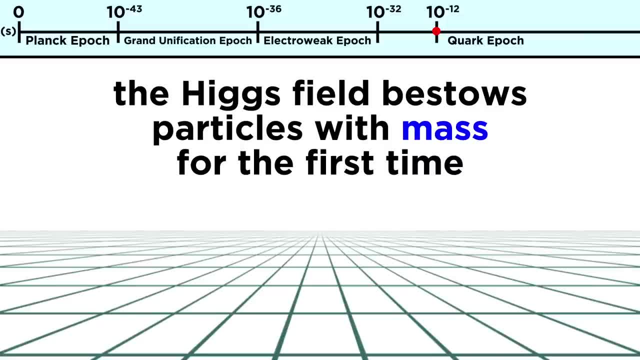 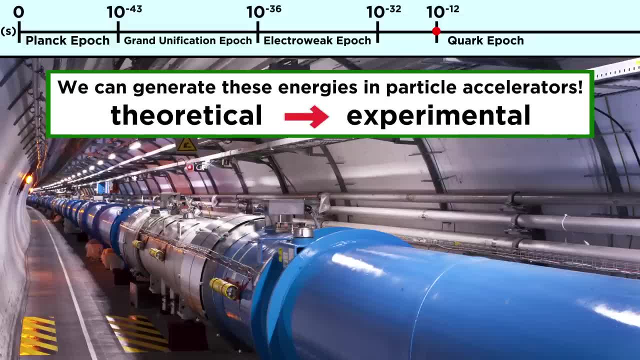 As a result, the Higgs field bestows existing particles with mass for the first time, but things are still too hot for protons and neutrons to form. This is also the highest energy epoch that we can currently probe with particle accelerators. 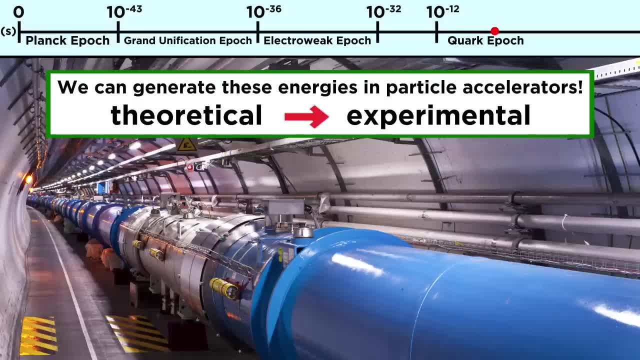 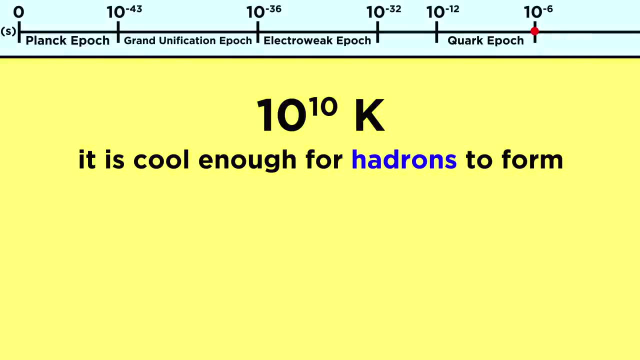 which means we are now transitioning from theoretical cosmology to experimental. At around ten to the negative six seconds after the big bang, things finally cool down. enough for the quark-gluon plasma that permeates the universe to congeal into hadrons, which 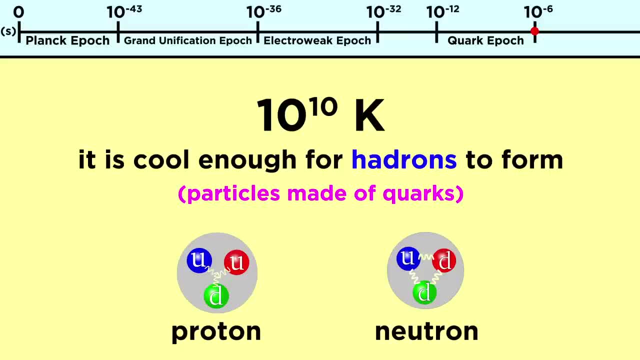 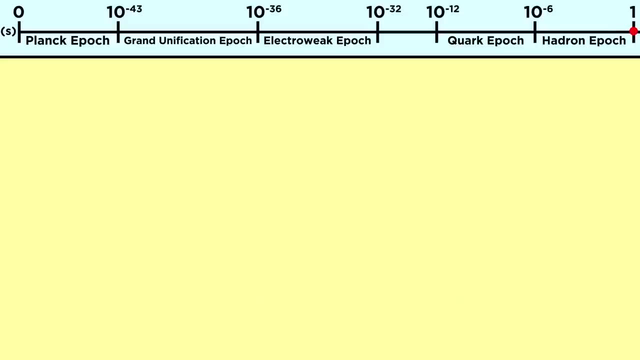 are particles made of quarks. This includes baryons like protons and neutrons, which will eventually make up all the atoms in the universe. This is called the hadron epoch, lasting until one full second. after the big bang, The action will slow down. 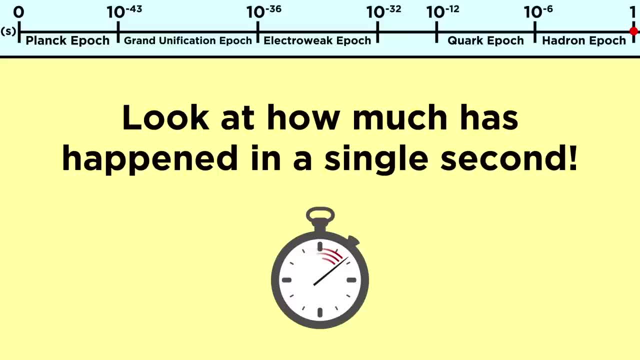 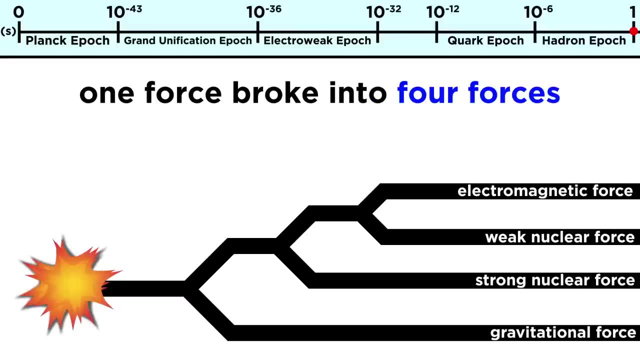 a bit from here, but before we move on, take a moment to imagine how much has happened in just one second: The void yielding merely some energy, and a singular force which sequentially breaks into four forces in turn, yielding a sea of massive particles. 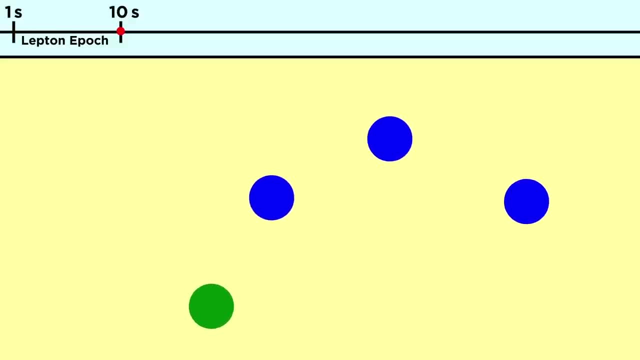 From one second to ten seconds after the big bang lasted the lepton epoch, Hadrons and antihadrons largely annihilate, leaving leptons and neutrons to be totally annihilated and antileptons to dominate, which in turn also largely annihilate. and thanks to a slight 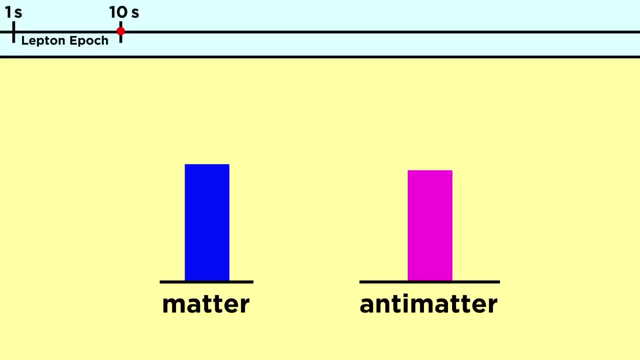 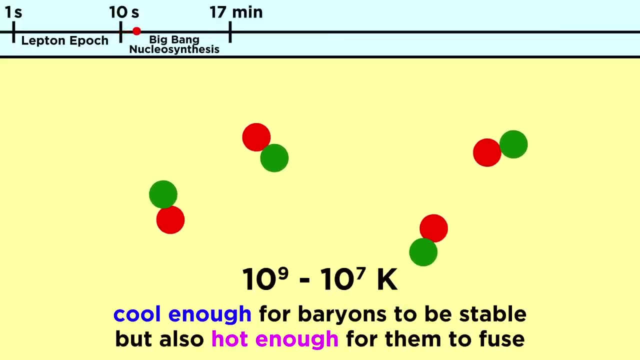 asymmetry in favor of matter over antimatter. this leaves just a fraction of the original matter behind. From here the start of the photon epoch. things start to look a little more familiar. For about seventeen minutes the universe is cool enough for baryons to be stable. but 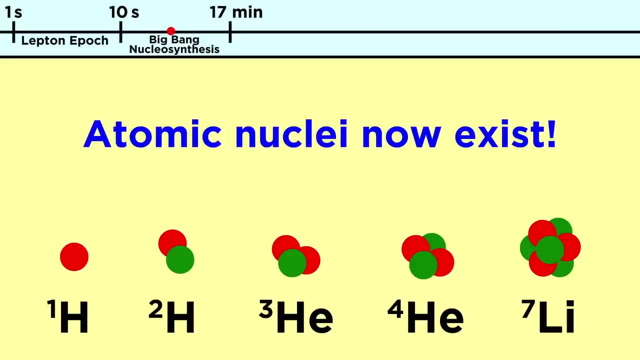 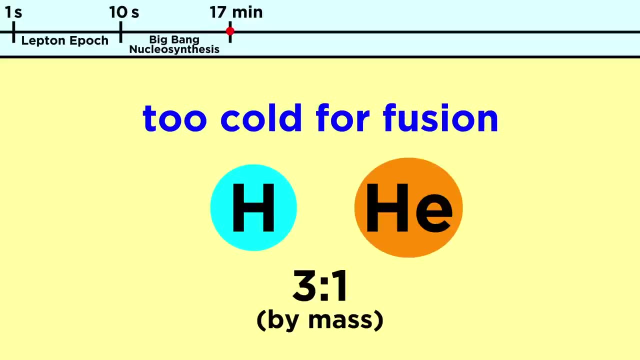 also hot enough for them to fuse. so protons and neutrons fuse together to make lots of hydrogen and helium and trace amounts of other light nuclei- an era called big bang nucleosynthesis. After that it gets too cold and sparse, so fusion halts, locking the universe into a 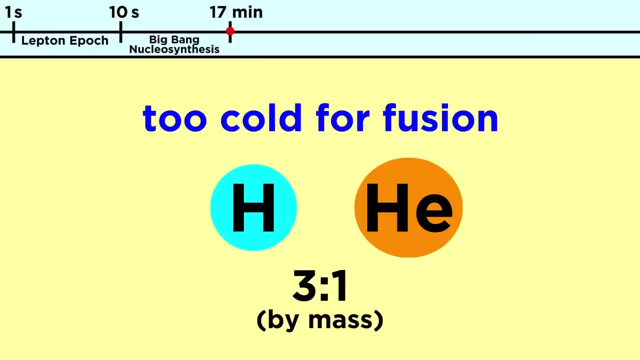 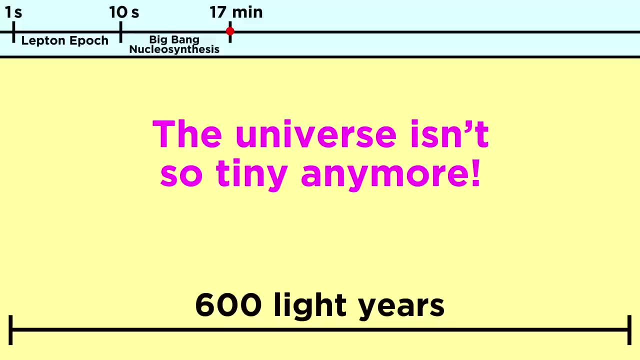 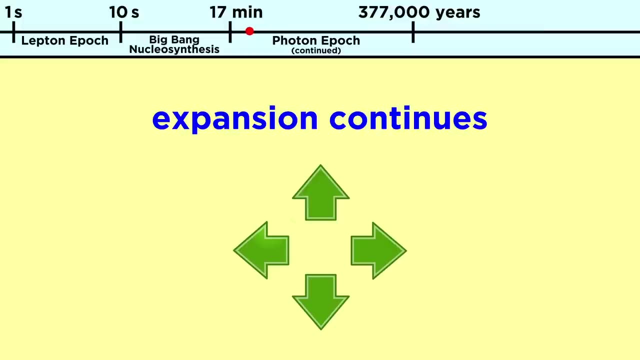 three to one ratio of hydrogen to helium by mass. At this point, the universe is about six hundred light years across, So we are no longer dealing with a tiny universe. Over the next several hundred thousand years, as the universe continues to expand, all of 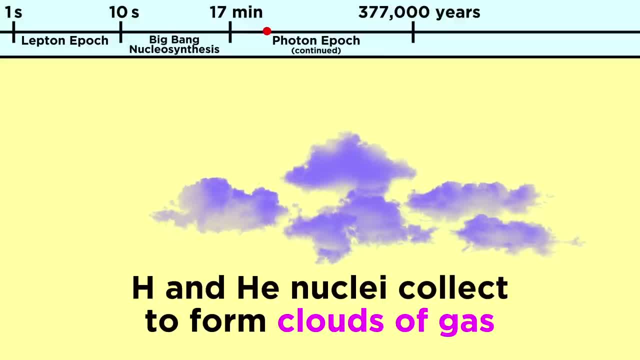 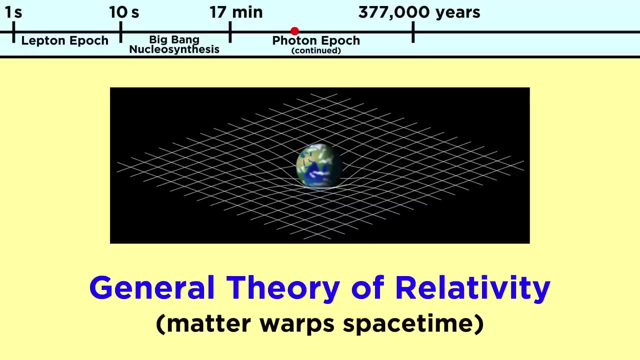 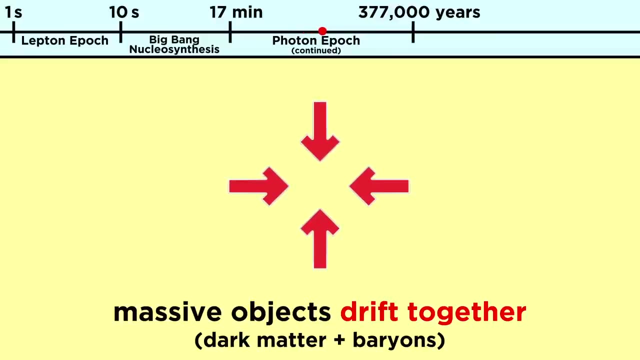 these hydrogen and helium nuclei begin to collect in little patches due to the effects of gravity. This force, now understood through Einstein's general relativity to be the warping of spacetime by massive objects, attracts all objects with mass towards one another. 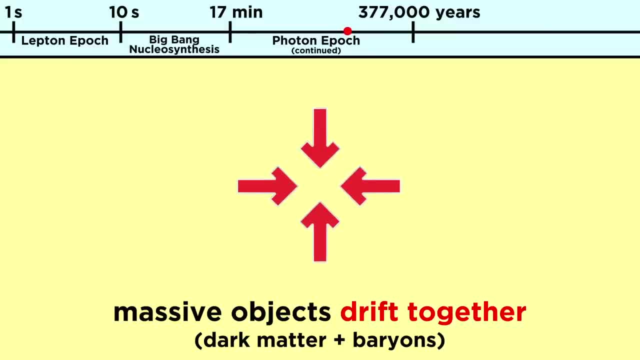 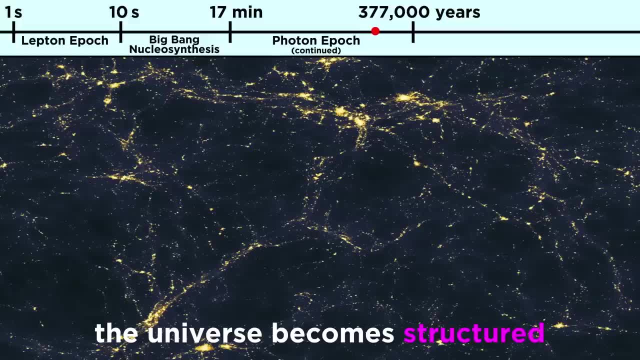 So, by virtue of the mass of these nuclei and more so all the dark matter around the universe which we will discuss later, the universe takes on a sinewy, filament-like structure. Denser regions become more dense and empty regions become more empty, as the photon epoch. 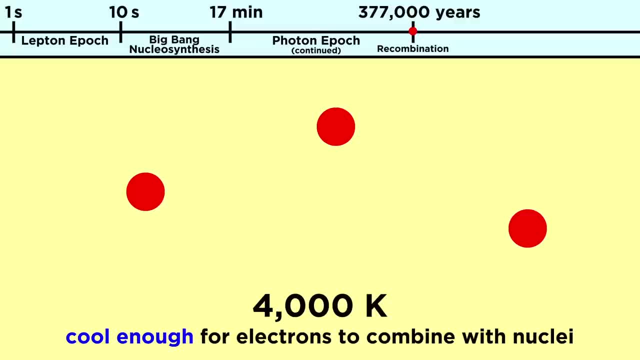 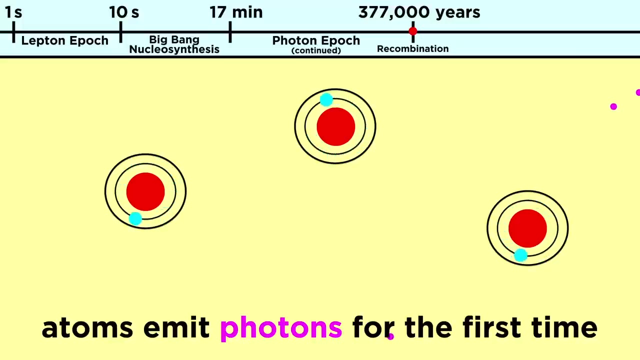 draws to a close During the next era, recombination and photon decoupling. about 377,000 years after the big bang, Things are finally cool enough for electrons to combine with nuclei to form neutral atoms for the first time. Electrons are captured, relax down to the ground state and emit photons in doing so. 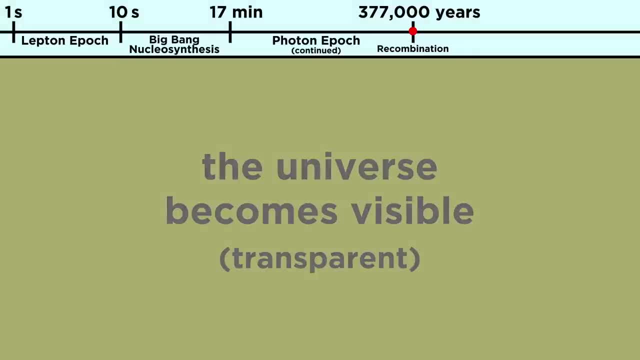 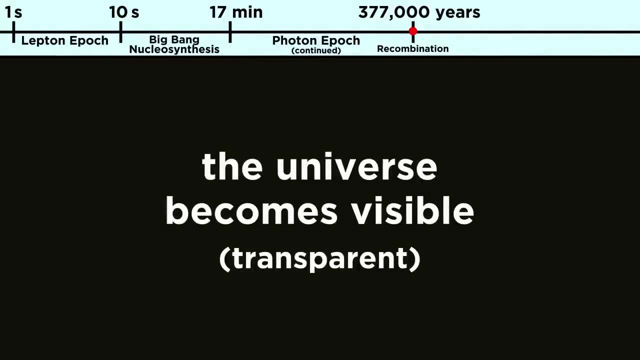 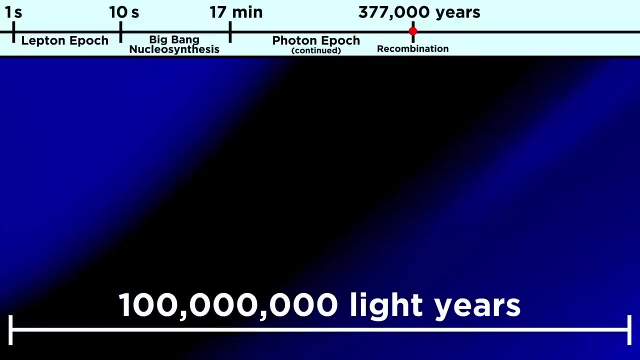 This marks the first time that the universe is actually visible, in the sense that we consider something to be visible to our eyes. It is no longer opaque but transparent, with electromagnetic radiation now moving freely over large distances and with a diameter for the universe of nearly 100 million light. 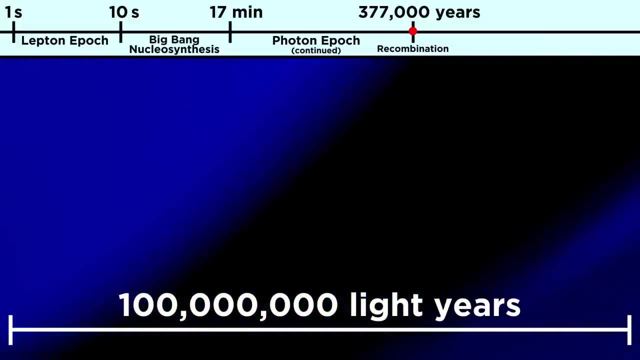 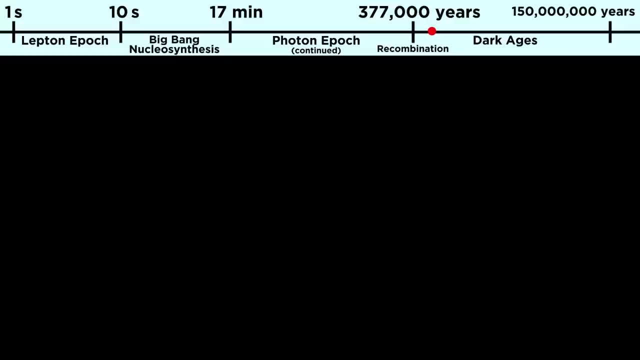 years. the distances are large indeed. Then, for around 150 million years, not much happened. We call this era the Dark Ages. There was plenty of hydrogen and helium around and photons were traveling everywhere, but there were no stars to produce all the light we see in the night sky today. 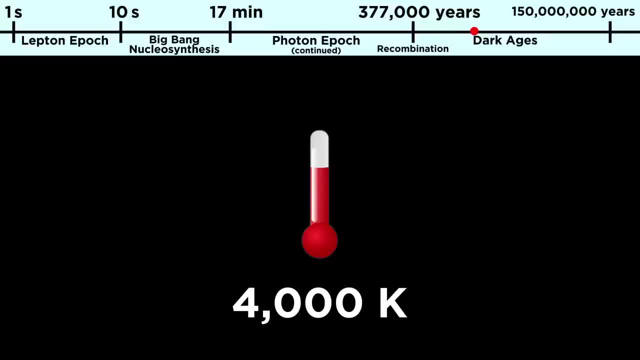 Things continued to cool From around 4000 kelvin down to 300 kelvin, which incredibly would allow for liquid water, if any were to exist, all the way to around 60 kelvin, a temperature that is finally cold enough by human standards to somewhat resemble the cold outer space we normally conceive. 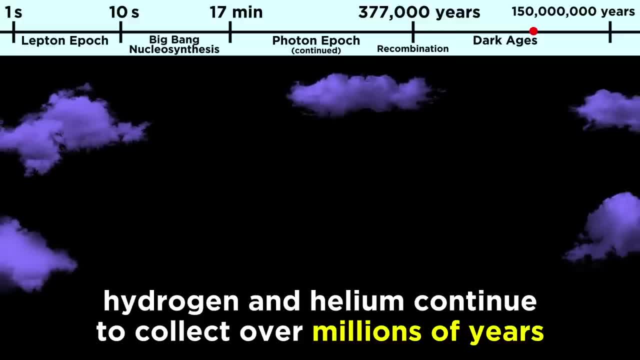 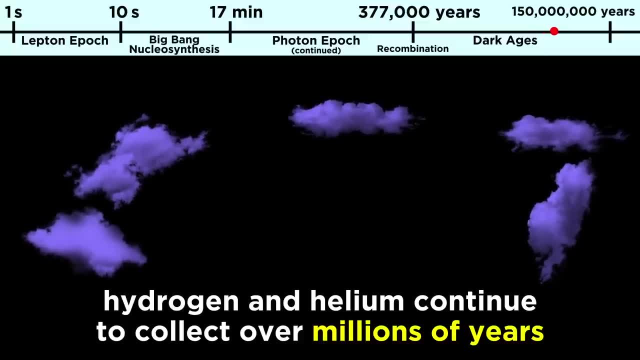 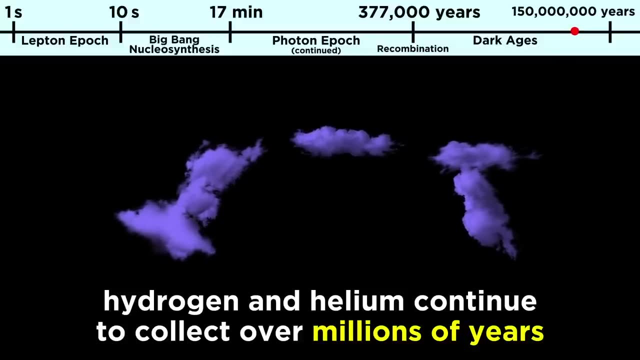 of, But slowly, ever so slowly. all the clouds of hydrogen and helium gas continue to collect Over millions of years. The minute gravity exerted by these particles, combined with the more significant gravity exerted by surrounding dark matter, pulled matter together into clumps little dense. 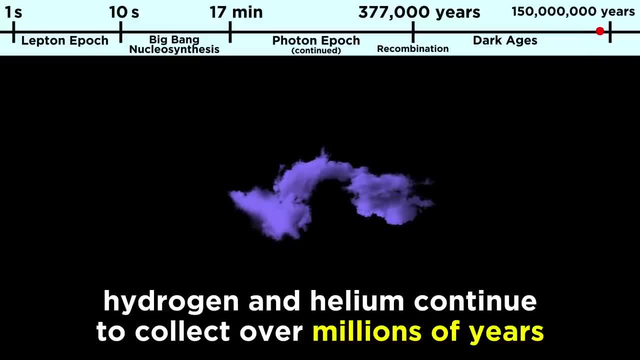 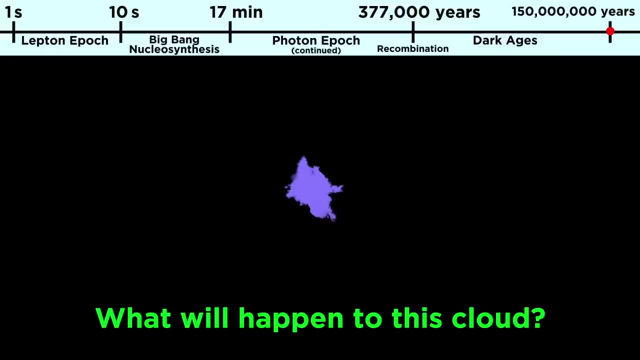 pockets of matter closer and closer, until all the atoms are pushing right up against one another. What happens when you get enough atoms all together in the same place- Ignition. So let's move forward and see what happened next. Thanks for watching, guys.